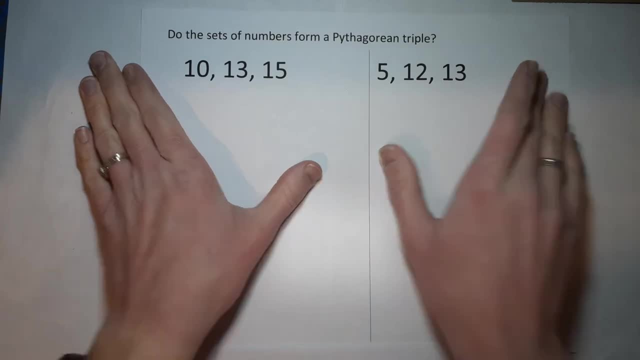 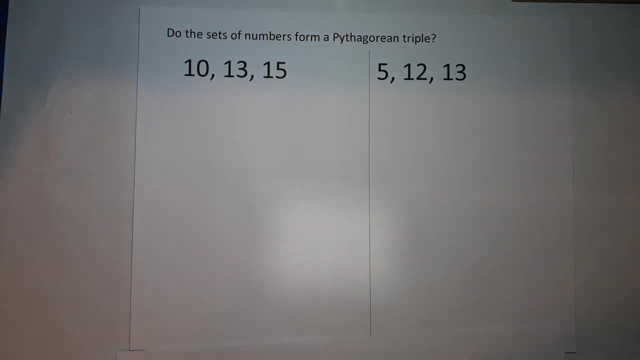 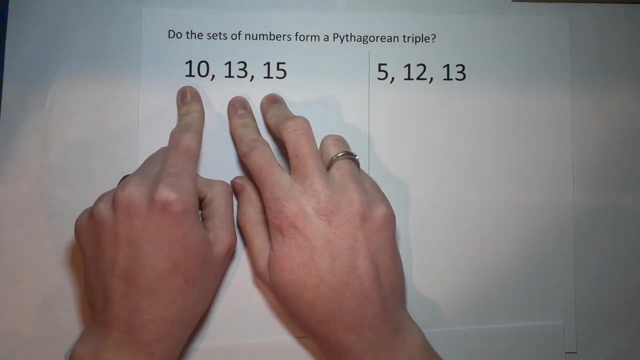 Pythagorean theorem if you need a bit more overview on that. But let's get started. Okay, they're wondering if this set of numbers 10,, 13, and 15 is a Pythagorean triple. So basically what they're asking is: could these be the sides of a right triangle? is basically what they're asking. 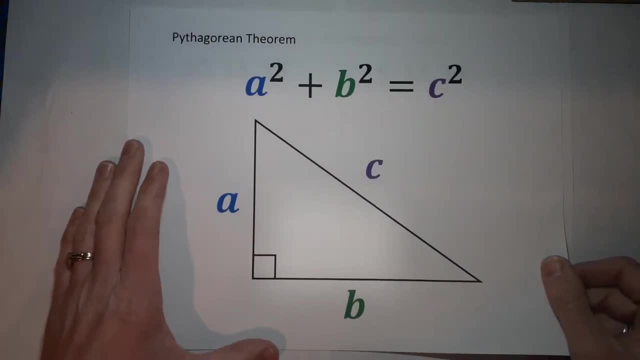 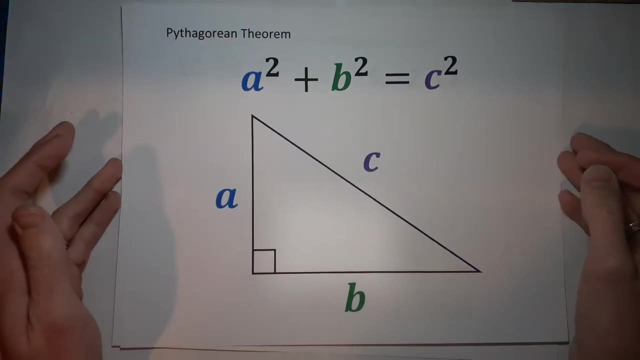 So Pythagorean theorem is what helps us determine if something can be a right triangle. Okay, a squared plus b squared plus c squared. I'm guessing you've probably been using it. Biggest thing to remember is that c is your hypotenuse. It's the long. 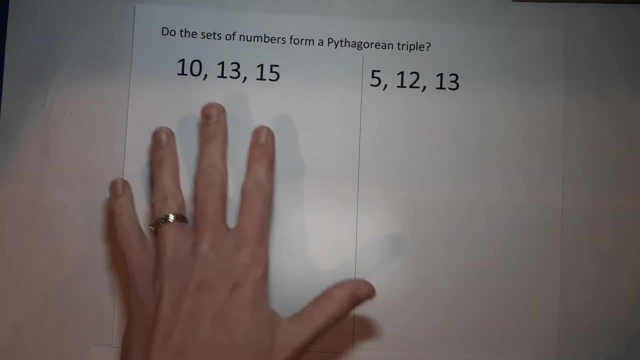 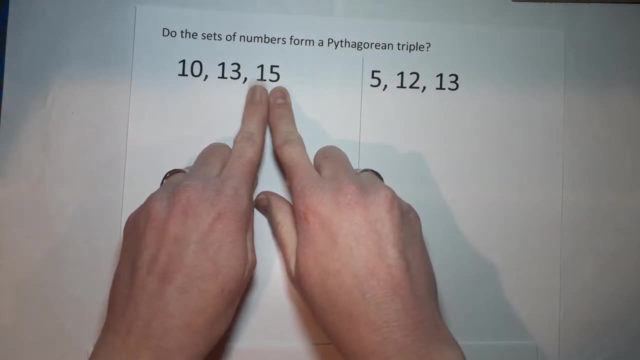 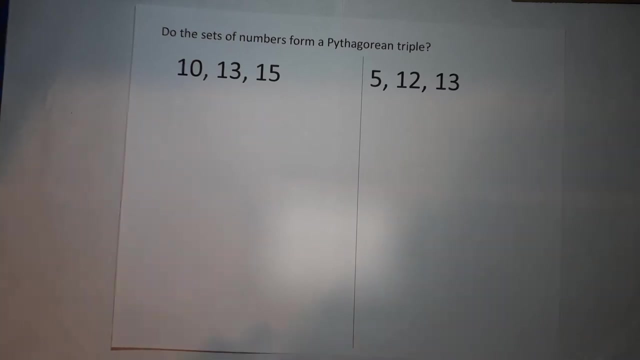 side. So in these examples we don't have the actual triangle with the sides labeled, but we know that the longest side, the biggest number, is the hypotenuse. if it is a right triangle- right. That's what we're trying to figure out is, if it is, if these could be the sides of a right. 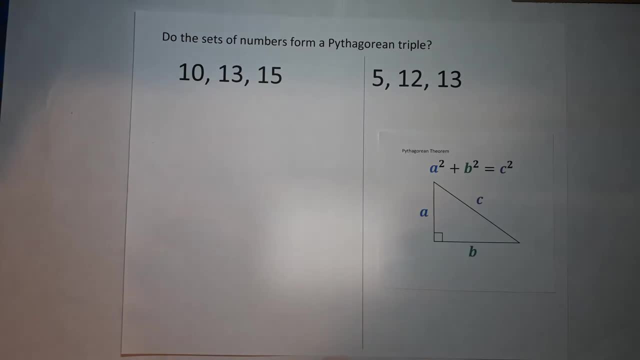 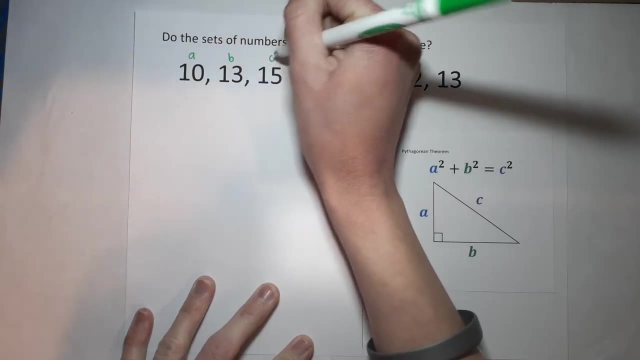 triangle. Okay, so here we go: 10,, 13, and 15.. So I'm going to label these as my a, b, and we know this one is c because it's the biggest, And b could be swapped, It doesn't really matter. Okay, so I'm going to set this up: 10 squared. 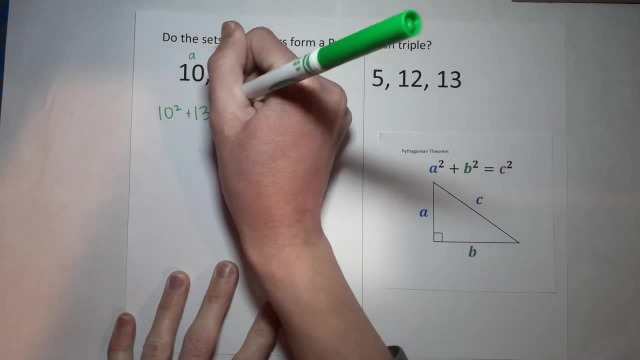 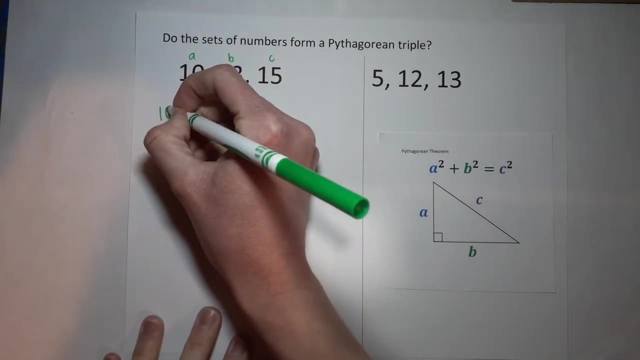 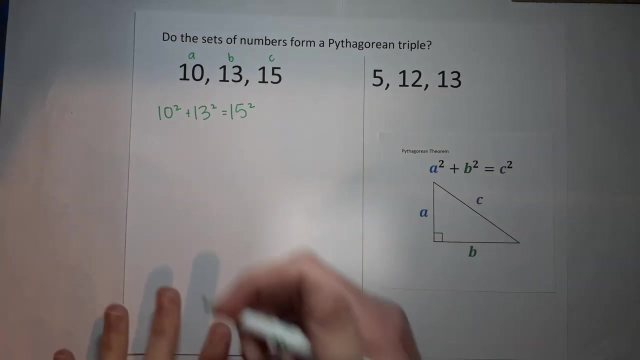 plus 13 squared equals 15 squared. Okay, and then we go from there: 10 squared, that is 10 times 10.. So it's not 20.. That's 10 times 2.. 10 squared is 10 times 10,, which gives me 100.. 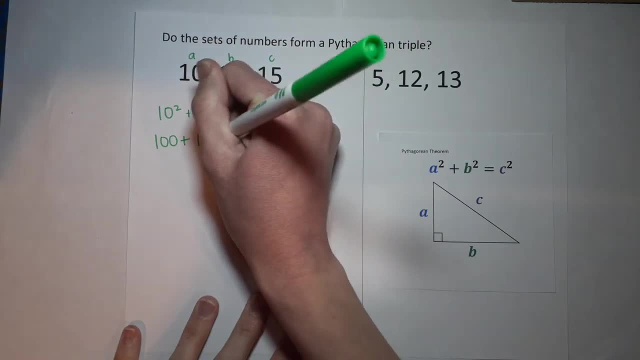 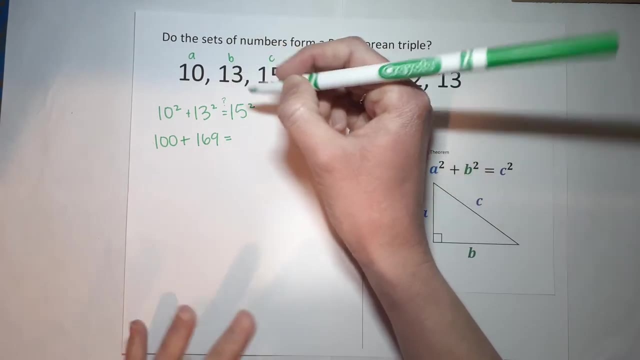 Plus 13 squared gives me 108.. 169.. I should put a little question mark here, because we're seeing if it's equal. We don't know for sure if it's equal or not, So we'll put that there. 15 squared is 225.. 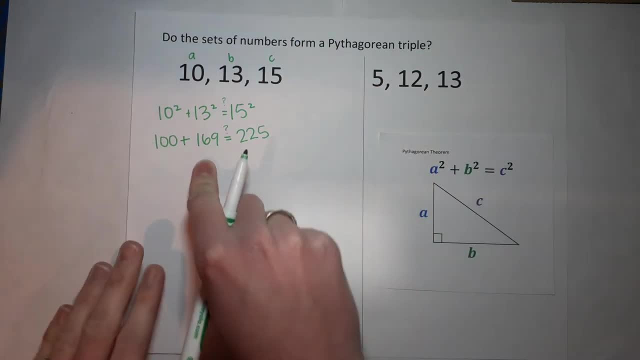 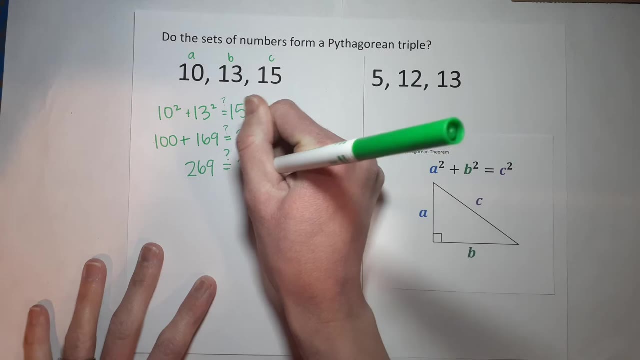 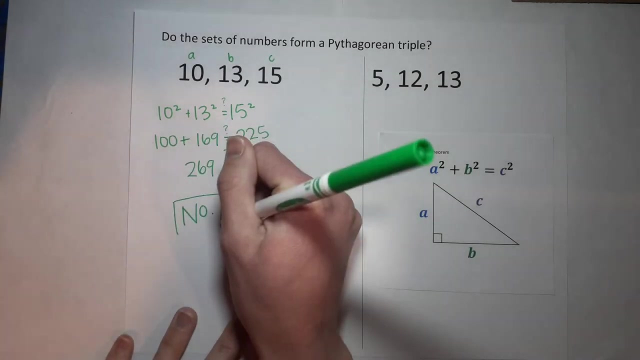 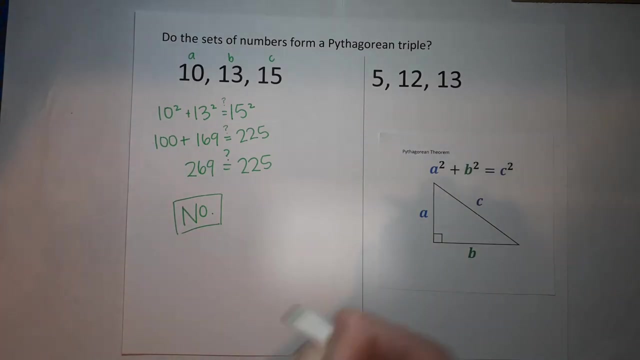 Okay, now 100 plus 169 is 269.. So does 169 equal 225?? No, Wow, That means this is not a Pythagorean triple. Okay, it did not work in the Pythagorean theorem, so it is not a Pythagorean triple. These numbers can tell us if it's a acute triangle or obtuse.